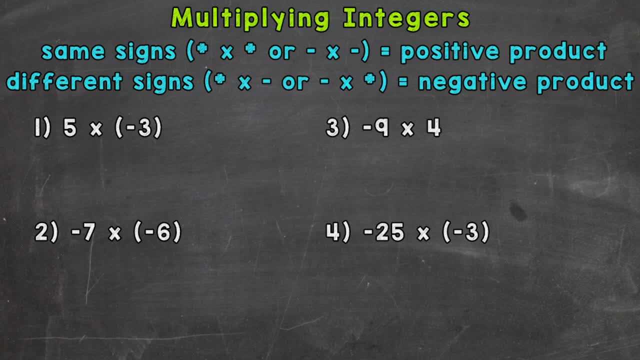 Let's jump into number one, where we have 5 times negative 3.. Now, at the top of the screen, we have some very important information when it comes to these types of problems. So if we have a multiplication problem where we have the same signs, 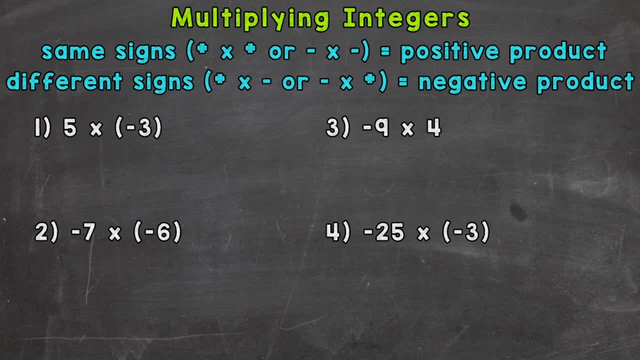 so positive times, a positive or a negative times, a negative, we get a positive product. Now, if we have different signs- so a positive times, a negative or a negative, times a positive- we end up with a negative product. So for number one, we have a positive times a negative. 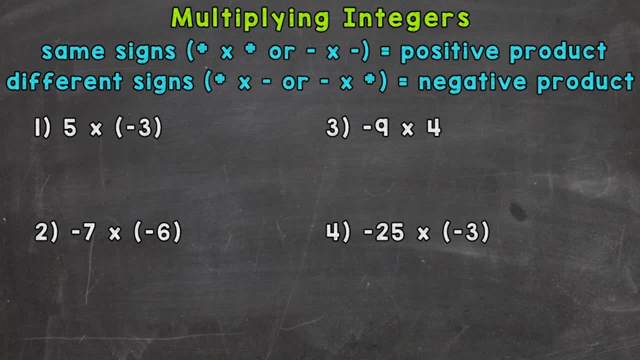 So different signs, that means we get a negative product. So we can do 5 times 3,, which is 15, and we know we had different signs, so a negative product. So our answer is negative 15.. Again, same signs equals positive product. 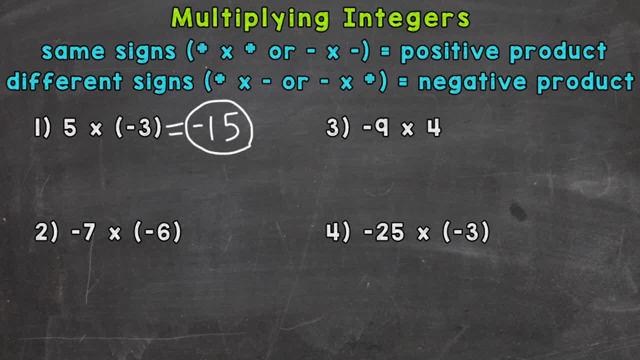 Different signs equals negative product. Let's take a look at number two, where we have negative 7 times negative 6.. Same signs equals positive product. We have two negative numbers there, So negative, Negative 7 times negative 6.. Well, 7 times 6 is 42, and we know that our product is going to be positive, so 42. 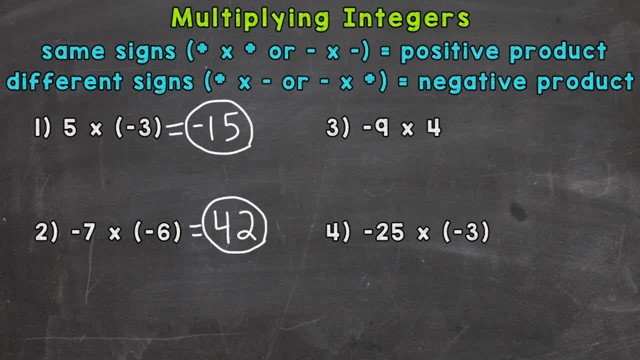 On to number three. So we have negative 9 times 4.. Different signs there. We have a negative times a positive. so we get a negative product. 9 times 4 is 36.. And, like we just mentioned, that's going to be negative. 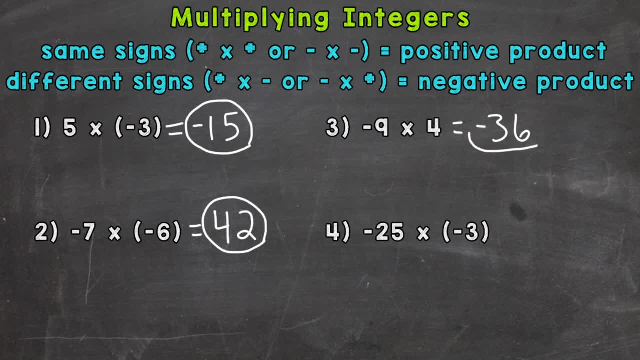 because we have different signs there. So negative 36.. And lastly, number four: we have a negative times a negative. So negative 25 times a negative 3. So same signs equals positive product. We know that 25 times 3 is 75.. 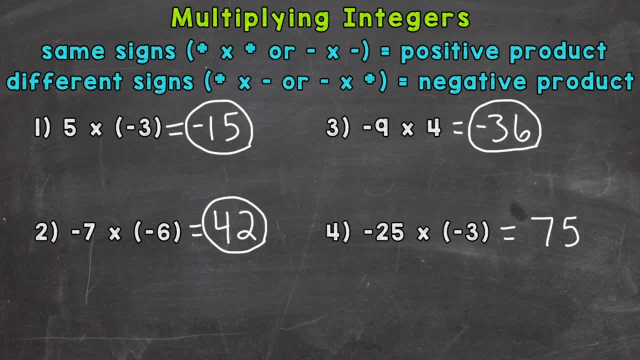 And, like we just mentioned, same signs equals positive product, We get a positive 75.. So there you have it. There's how you multiply integers. Remember: same signs equals positive product, Different signs equals negative product. I hope that helped. 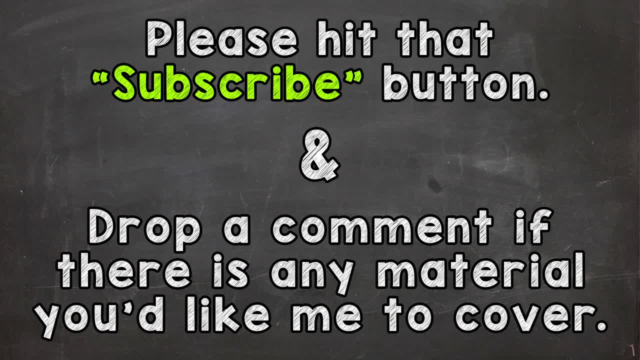 Thanks so much for watching. Until next time, Peace.